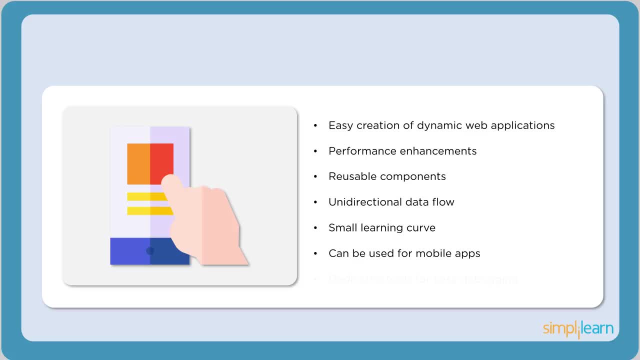 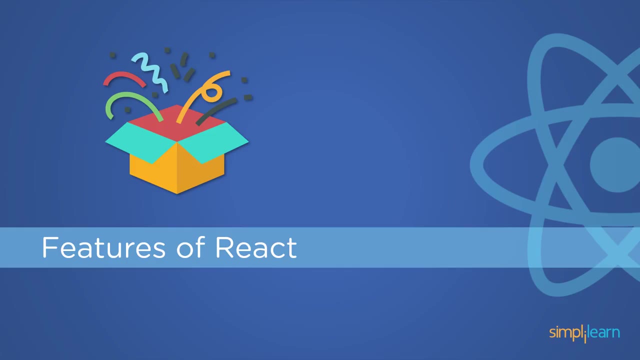 React is much easier to learn. React recently released an extension called React Native that is used for developing mobile applications that are cross-compatible. It also has dedicated tools for easy debugging. Now let's dive in to the features of React. First, let's understand JSX. JSX is a syntax. 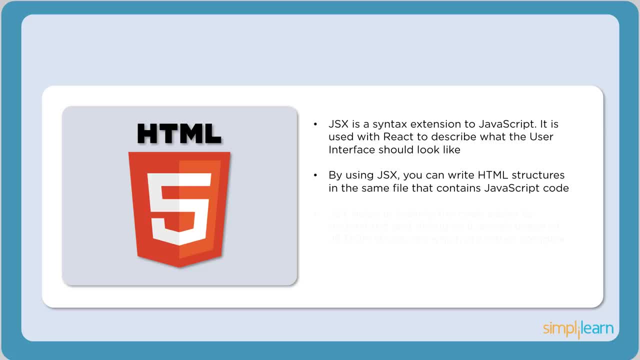 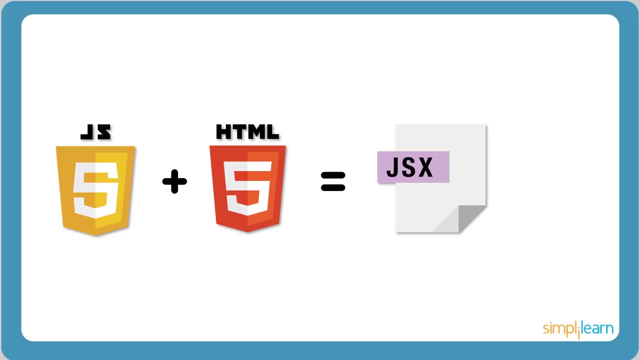 extension to JavaScript. Using JSX, we can add HTML to the JavaScript file. All coding in React is done using JSX. It also helps in making the code easier to understand. We can also use JSX to understand and debug. Ultimately, JSX is a combination of JavaScript and HTML. Now let's 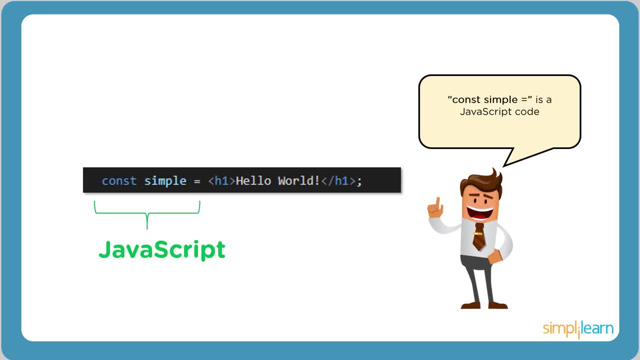 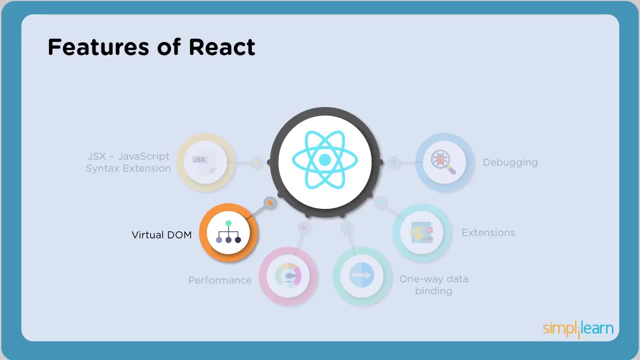 consider a small example. Const simple. here is a JavaScript notation. H1 tags indicate HTML. Again, the semicolon indicates JavaScript. Note that the semicolon is not mandatory. However, it's a good practice to include it. Moving on, the next feature is virtual DOM- DOM, which is an acronym for data object model. 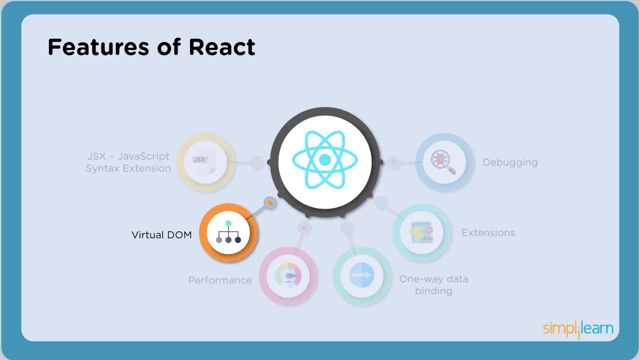 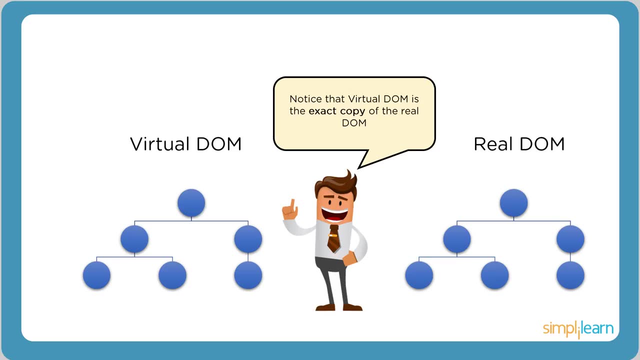 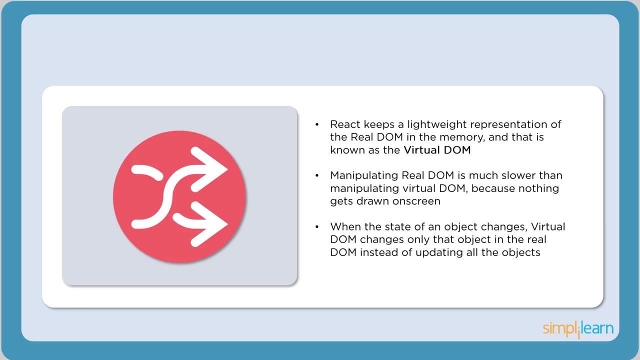 actually defines how documents and files are structured. This is a key feature we'll talk about in the next video. Now let's see how this actually works. React creates a virtual DOM that is the exact copy of the real DOM. Traditionally, whenever something changes in the web application, all objects 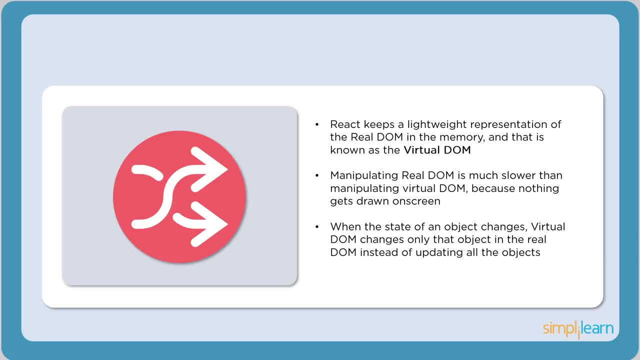 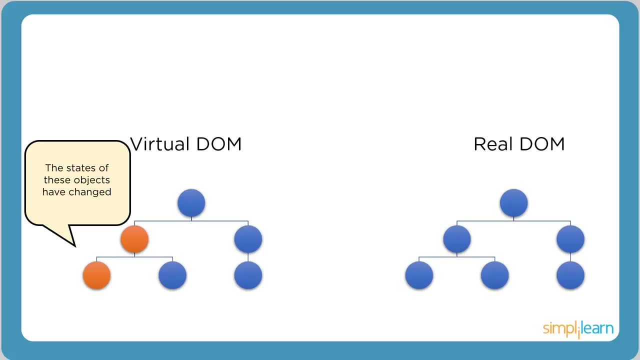 in the real DOM are updated. This makes it extremely slow. Let's see how React counters this. Now consider two objects whose states have been changed. React now compares the virtual DOM with the virtual DOM snapshot. that was taken right before the update By. 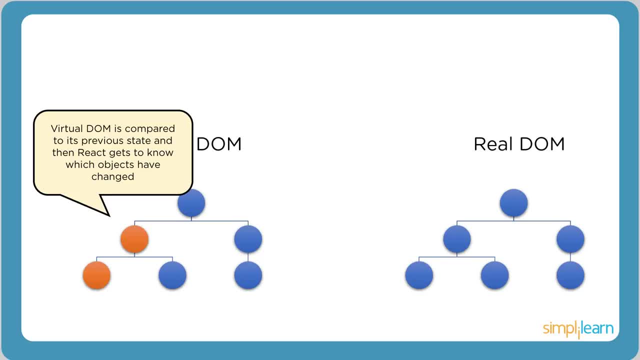 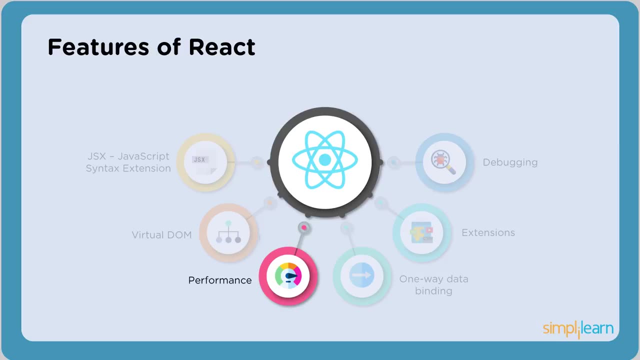 comparing the new virtual DOM with the pre-update version, React figures out exactly which virtual DOM objects have changed. Now React only updates those objects on the virtual DOM. This makes a big difference when it comes to speed. Coming to the next feature, performance. React uses virtual DOM, As discussed earlier, virtual 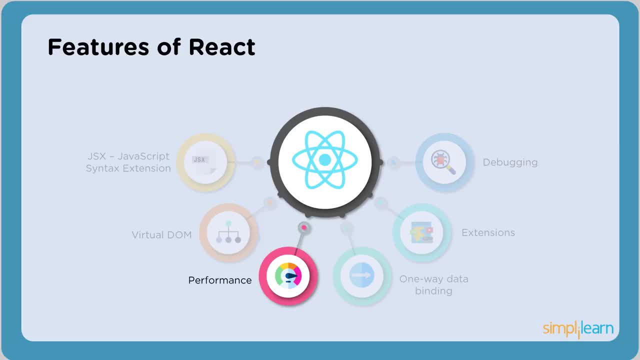 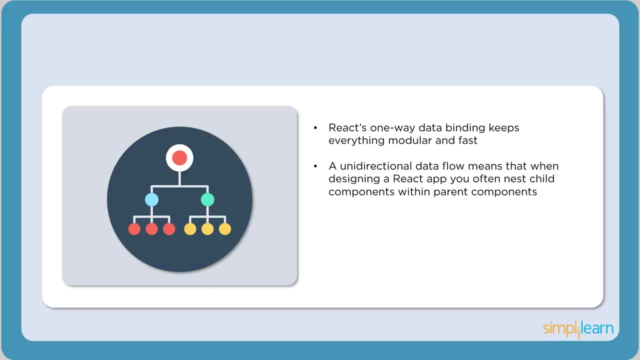 DOM impacts the speed of the web applications. We also took an example of Instagram and learned how multiple components can affect the development time. They help improve performance drastically. The next feature is one-way data binding. This means information flows in only one direction. One-way data binding is specifically used when information is displayed and not 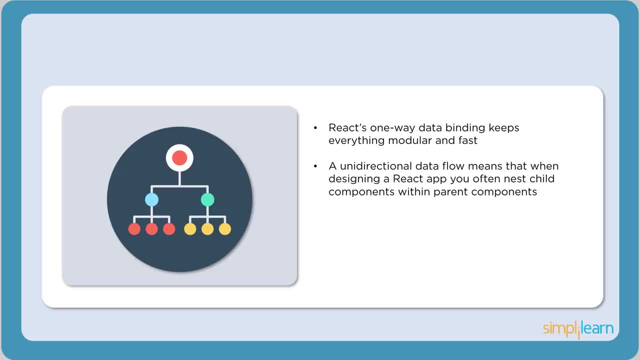 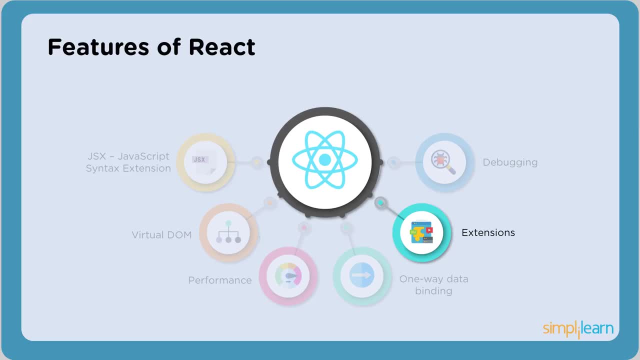 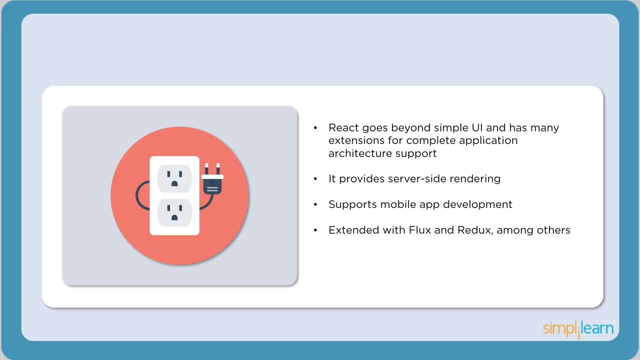 updated. Remember that the components of React are functional in nature, That is, they receive information through arguments and pass information via their return values. The next important feature is extensions. React has many extensions that we can use. React provides server-side rendering, which means that the application is rendered on 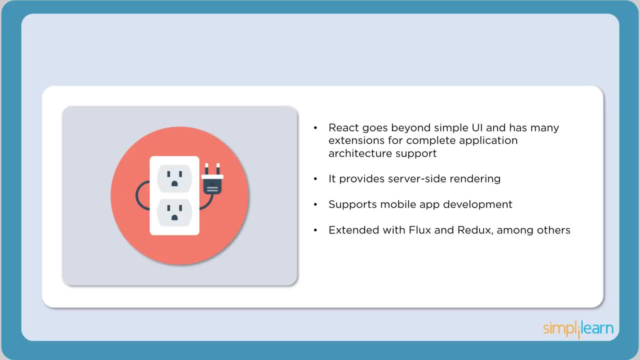 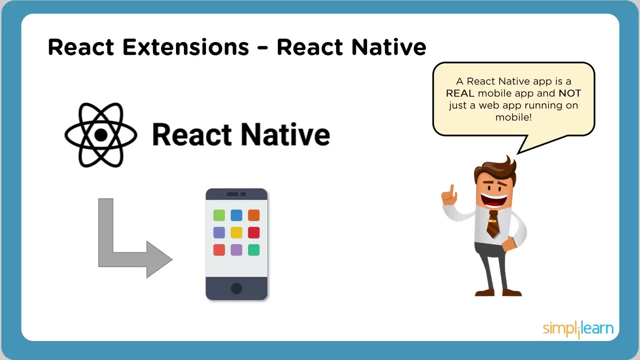 the server rather than in the browser. React Native, which is a React extension, is used for developing mobile applications. There are many other extensions that React provides for every scenario in web development. Let's look at a few of them. React Native lets you build mobile applications using only JavaScript. A React Native app is: 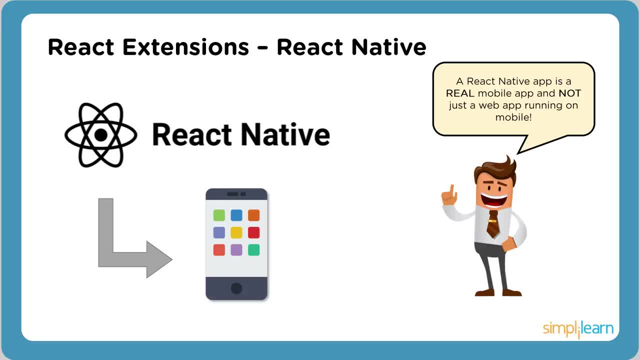 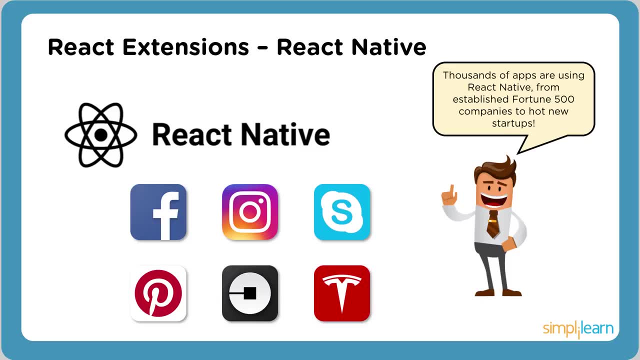 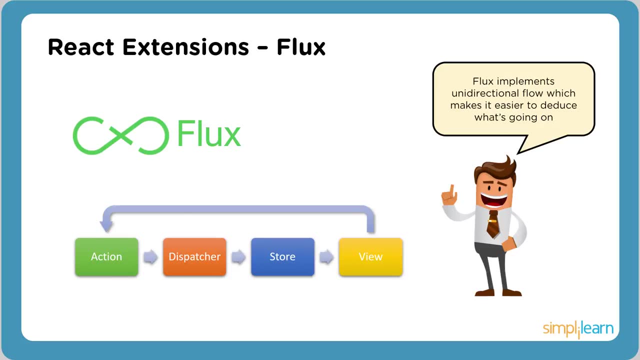 a real mobile application and not just a web application running on your mobile devices. Thousands of applications like Facebook, Instagram, Pinterest, Skype use React Native. The next popular React extension is Flux. Flux is the application architecture that Facebook uses. Flux implements a unidirectional flow, which makes it easier to understand what actually. 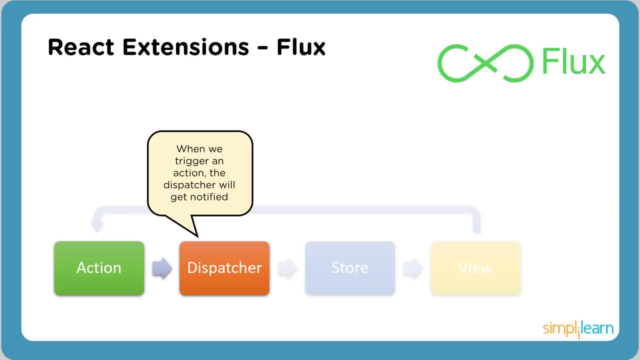 is going on. Now let's see how it works. When we trigger an action, the dispatcher will get notified. The dispatcher receives actions and dispatches them to the stores. A store is what holds the data of an application. Stores will register with the application's dispatcher so that they can receive actions. 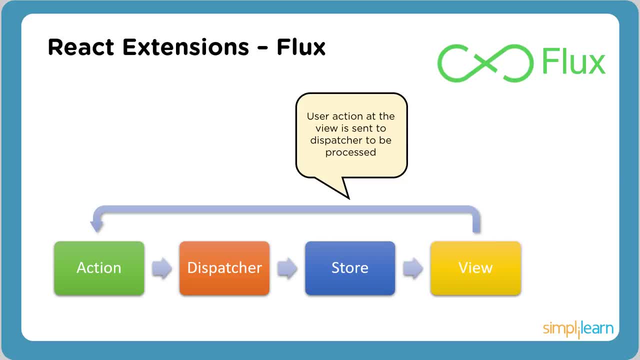 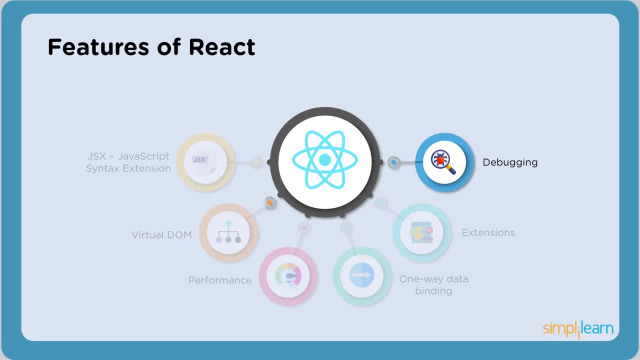 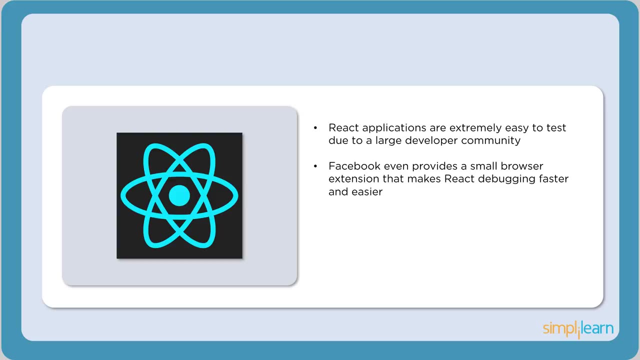 Data from stores is displayed in views. Actions define the internal API of your application. They capture how anything might interact with your application. The last feature of React is debugging. React applications are easy to debug thanks to the large and active developer community. You can practically debug React codes within your browser. 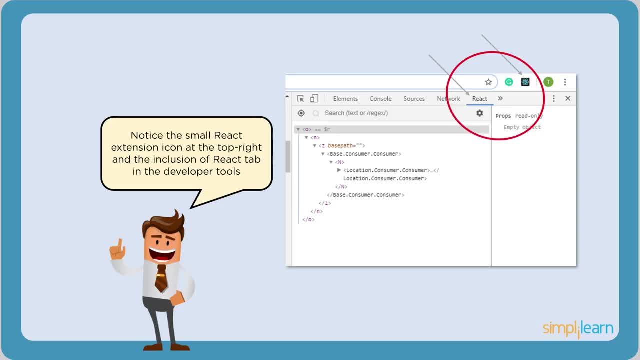 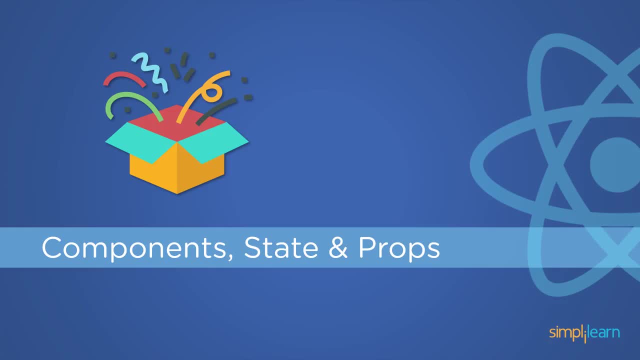 Now notice the small React extension icon at the bottom. This developer tool allows the user to inspect the code and also easily debug it. Moving on, let's learn about the building blocks of React. Components, state and props are the essential concepts that one should know before implementing. 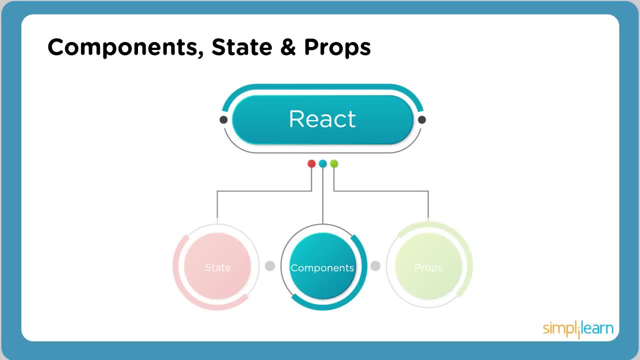 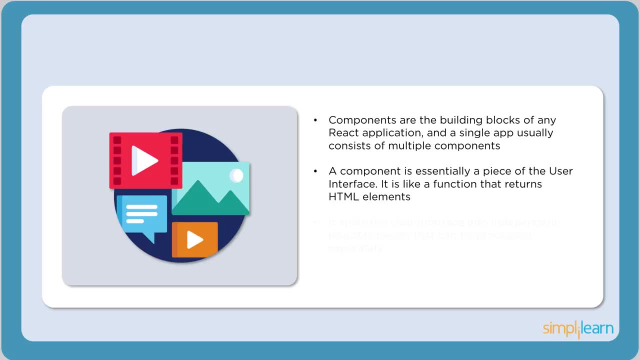 React. They are the foundation on which React is built. Now, what exactly are React components? Components are the building blocks of any React application. React divides the user interface into multiple components, wherein each component defines how a particular element is viewed in the application. 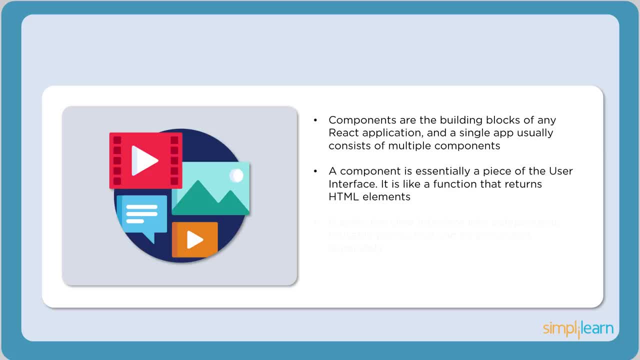 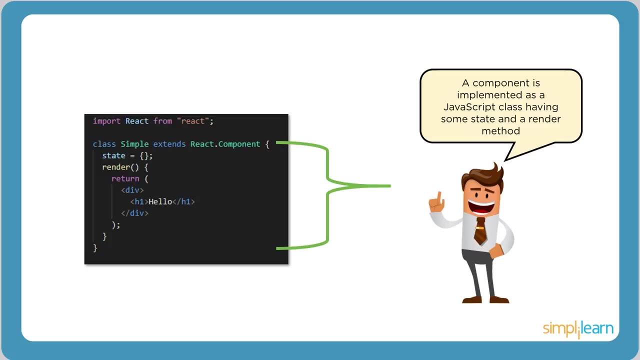 React components remain discrete and are processed independently. Another feature is reusability. Components can be reused multiple times across the application. This reduces the development time. Consider the following code snippet: A component is implemented as a JavaScript class having some state and a render method. 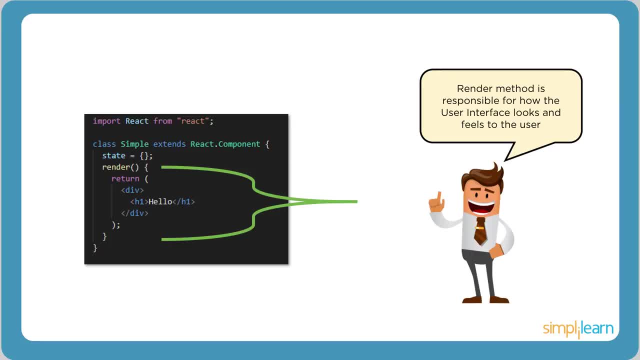 State is the data which we want the component to render. The render method is responsible for how the UI looks and how it looks in the application. The component is the data which we want the component to render. The render method is responsible for how the UI looks and how it feels to the user. 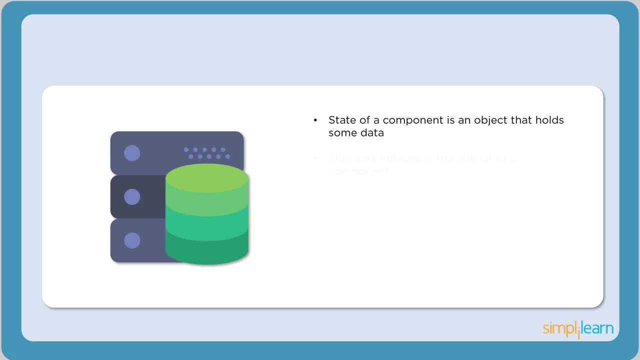 The next concept is state. State of a component is an object that holds some data. This data influences the output of a component. Every time the state of an object changes, the component is re-rendered onto the screen. Now let's see what props are. 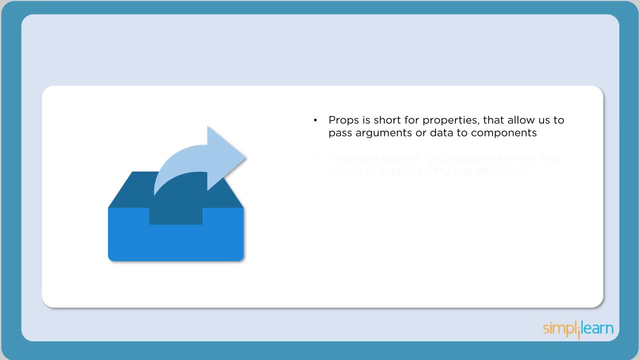 Props, or short for properties, allow us to pass arguments or data to components. Properties help make components more dynamic. It is important to define all the properties, their types and their default values. It is important to define all the properties, their types and their default values. 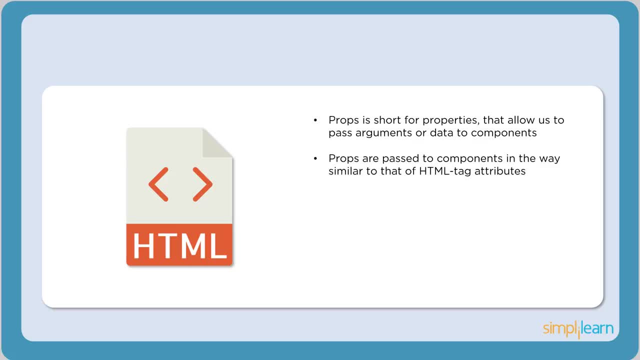 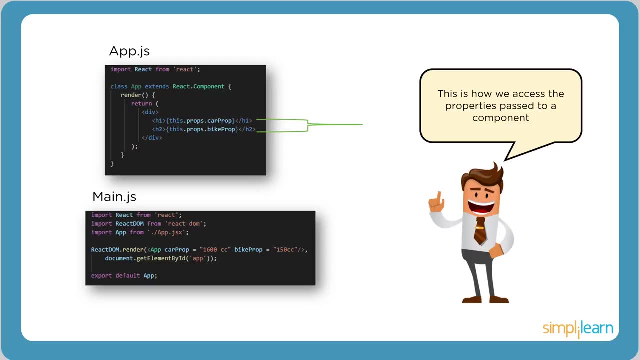 Also, props are passed to components in a way similar to that of HTML tag attributes. Now consider the following code snippets. This shows exactly how properties are passed to components. Also, detailed illustrations on components, props and state will be shown in in upcoming videos, So stay tuned for that. 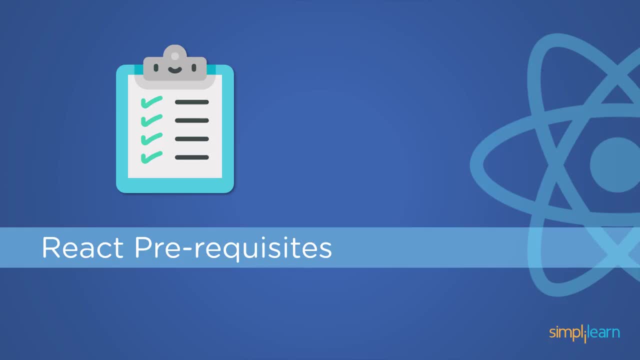 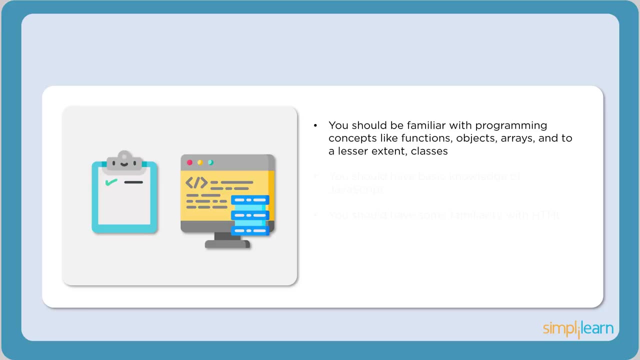 Moving on, let's go through some of the things that you should know before you can actually start working on React. You should be familiar with programming concepts like functions, objects, arrays andін classes. One should also have a basic knowledge of JavaScript and a familiarity with HTML. 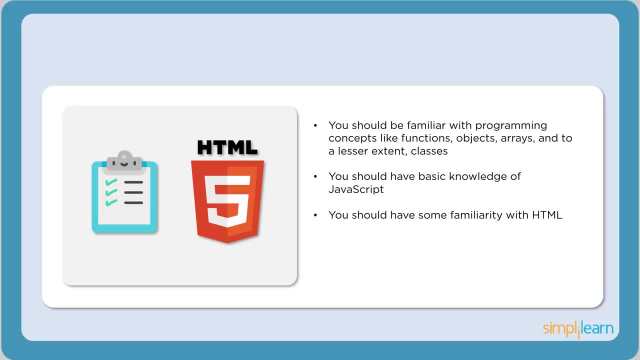 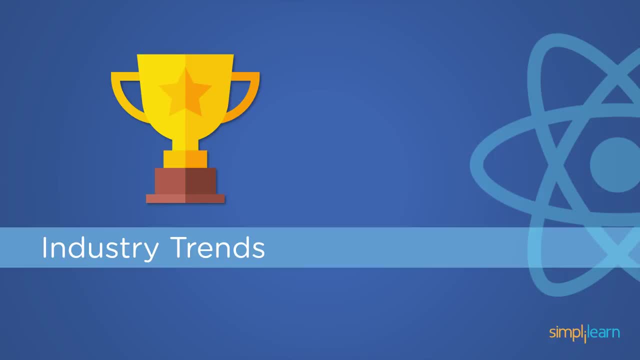 Don't worry if you feel like you're not good at them. Once you start working on them, you'll get a good hang of it. Finally, let's go through the impact of React on the IT industry and get insights into the salaries of React developers. 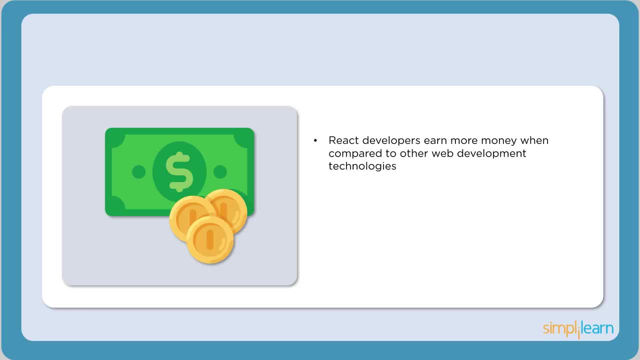 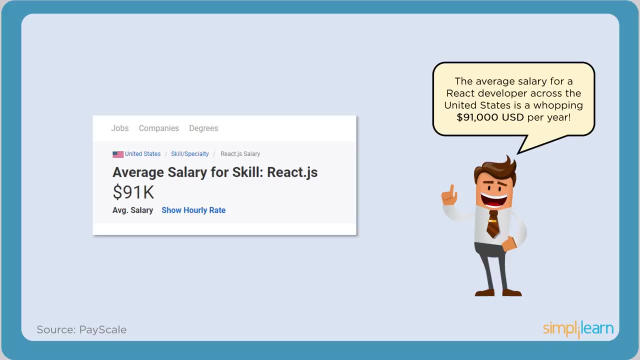 Statistics show that React developers earn way more than other web developers. According to PayScale, the average salary for a React developer in the United States is a whopping US$91,000.. The average salary for a React developer in India is 7.25 lakhs per annum. 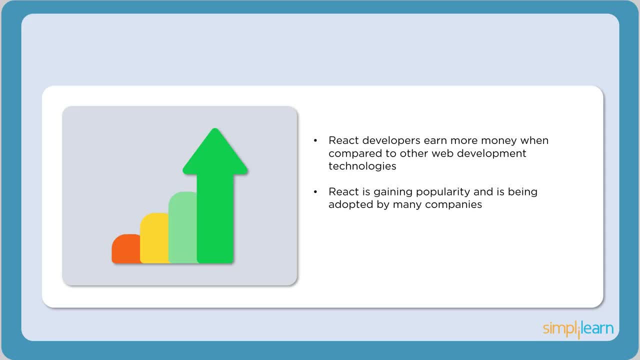 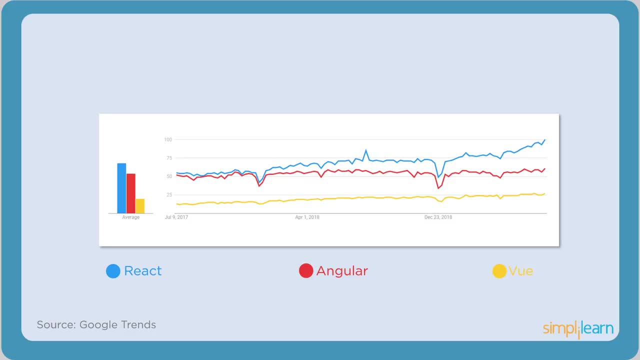 Over the recent years, React has gained immense popularity and is being adopted by many companies. According to the data by Google Trends, React has had a better growth scale compared to other frameworks like Angular and Vue. Statistics show that front-end developers have wholeheartedly